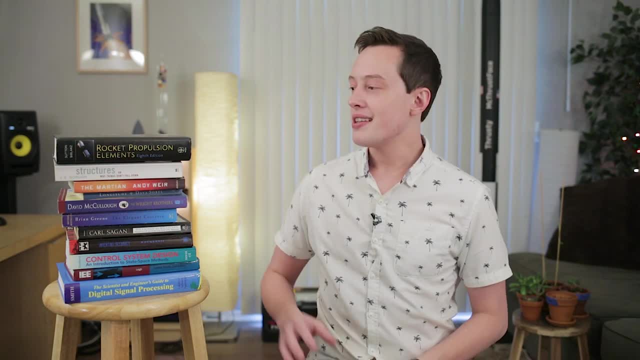 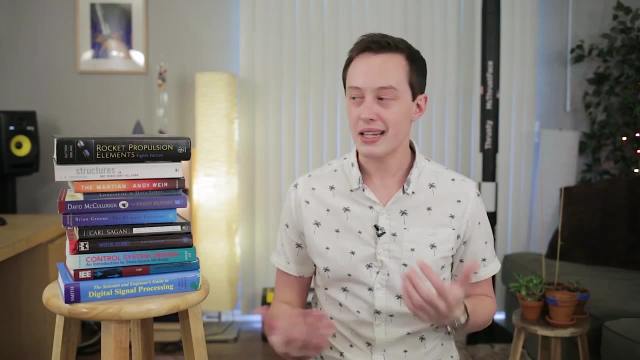 you should read. There's no one list that works for everyone. These are just the books that I have personally read and that I can personally vouch for. There are plenty of other texts that you should read if you're interested in getting started with this stuff. 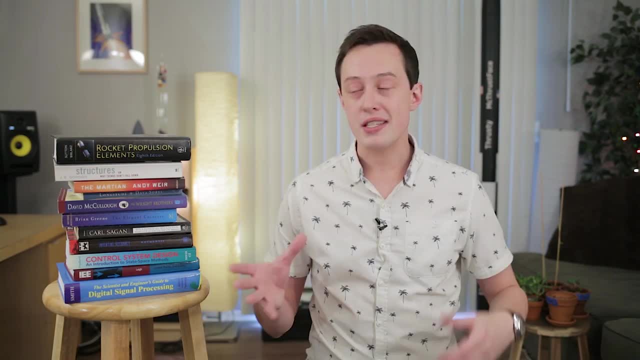 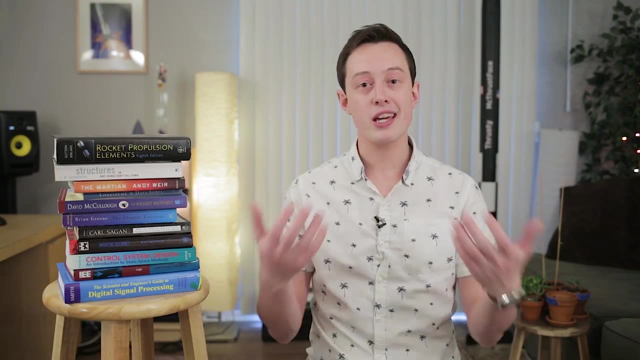 but these are the ones that had the biggest impact on me. Another caveat is that I will be providing links to all of these books in the description, but the links are affiliate links, which means that BPS and I get a small kickback from Amazon when you purchase using 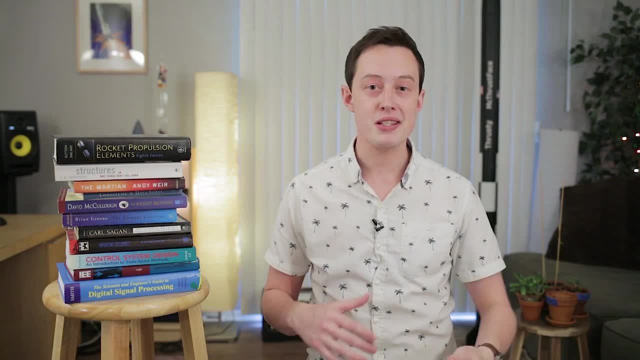 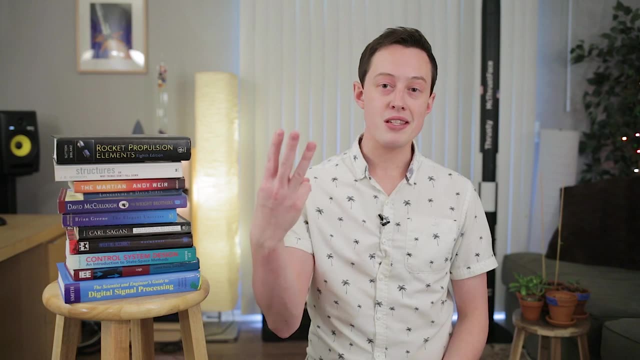 those links. You don't have to do it, but I just want to be transparent about when stuff is sort of sponsored or you know things like that, You get it. And the final thing to note is that I'm breaking this video up into three separate sections. The first section: 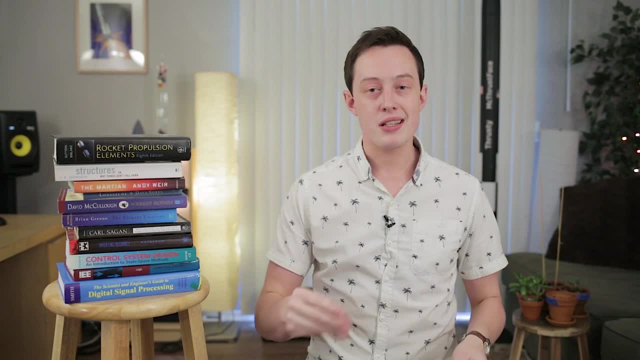 is just going to be books that are more technical and textbook-y. The second section is books that are sort of focused on engineering and they're easy reads with minimal math, but they're also books that are more technical and textbook-y. The second section is books that are sort of focused on engineering and they're easy reads with minimal math, but they're 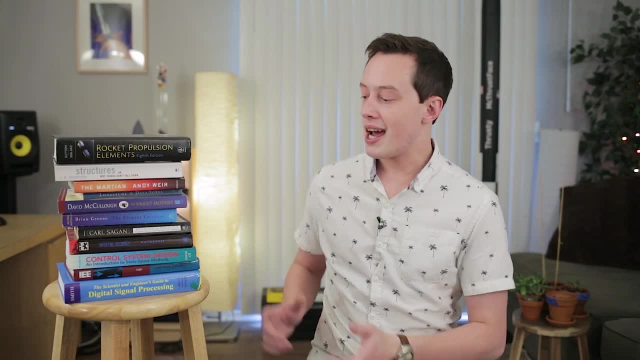 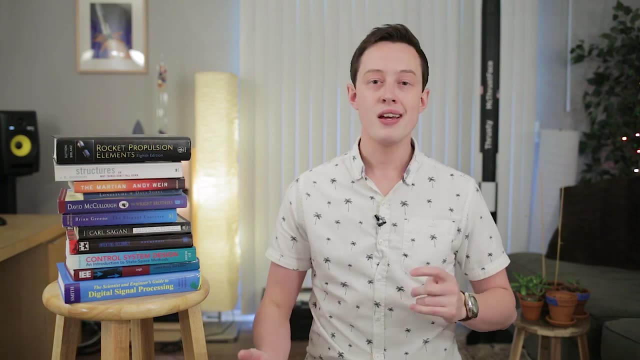 also books that are sort of focused on engineering and they're easy reads with minimal math, but they're also not textbooks, they're not directly going to help you. And the third list is books that I am currently reading. so while I can vouch for them, I haven't finished them or I haven't gotten far enough where I can say: 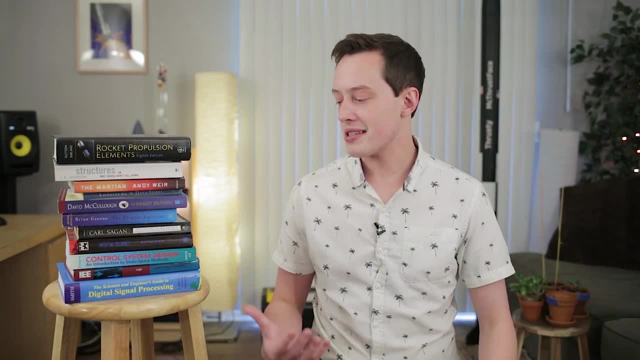 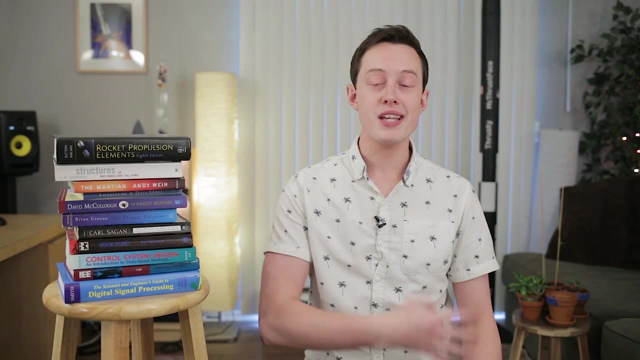 they're, you know, excellent. I hope that doesn't count against them. It's just books that I'm currently reading. if you're interested in following along with that, There's also a fourth list of books that's going up on the second channel, linked down below, and 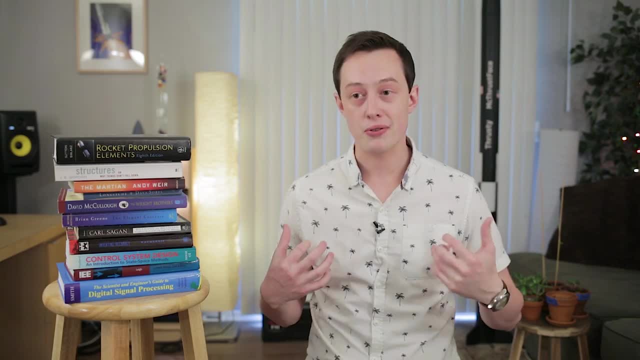 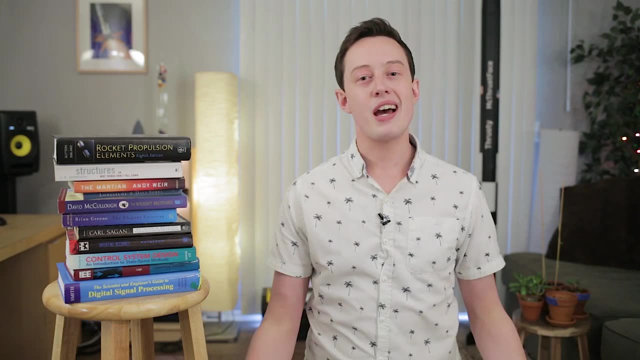 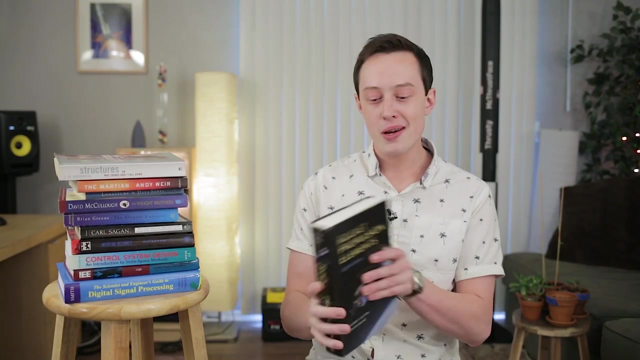 these are books that I personally have found helpful for like personal growth- So not engineering related, nothing like that- although they are mostly still focused on engineering. So with all that out of the way, let's get started with our first book, which is Rocket Propulsion Elements. This is so. 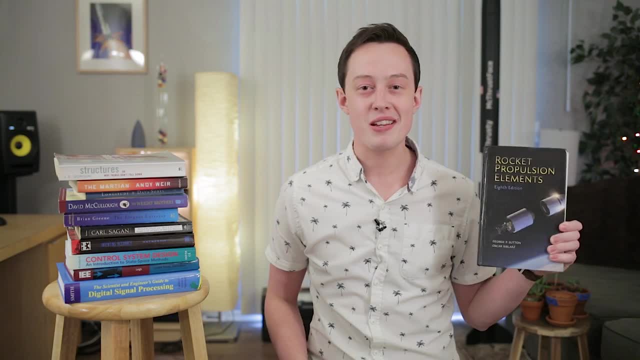 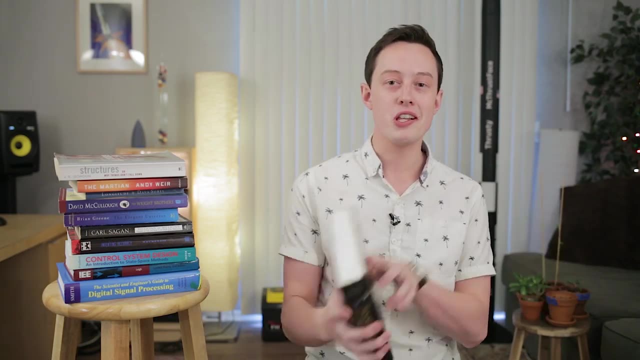 predictable. So this is a classic aerospace engineering textbook especially. I feel like I just don't have to describe at all what it is. It describes rocket propulsion elements. So looking through it, just flipping through it a little bit, here we've got diagrams of what looks. 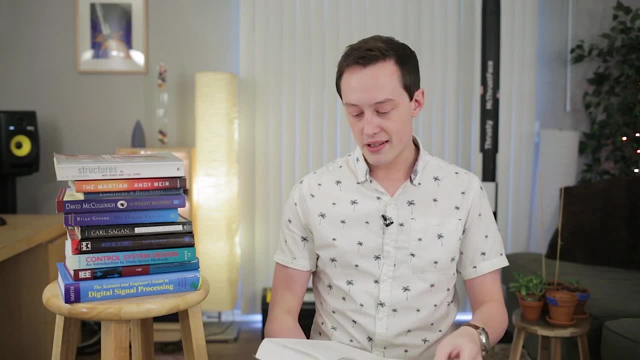 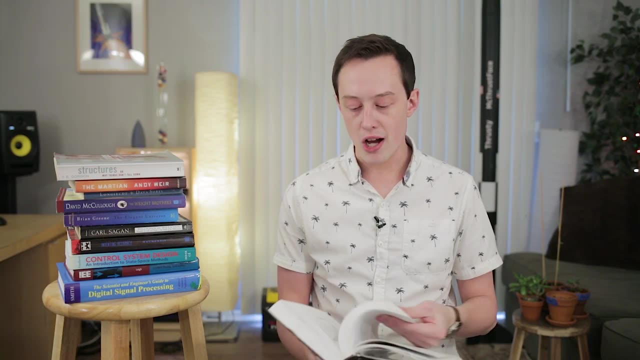 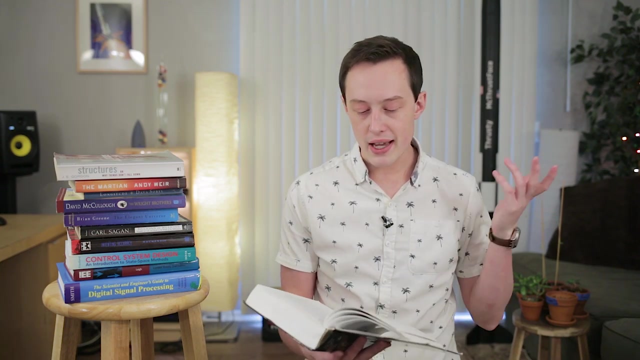 like maybe a SSME. We've got charts about different types of energy from different types of fuel. This is basically a really it's a comprehensive guide to propulsion in modern rocketry and some past stuff as well. Now, this hasn't actually helped me that much directly in. 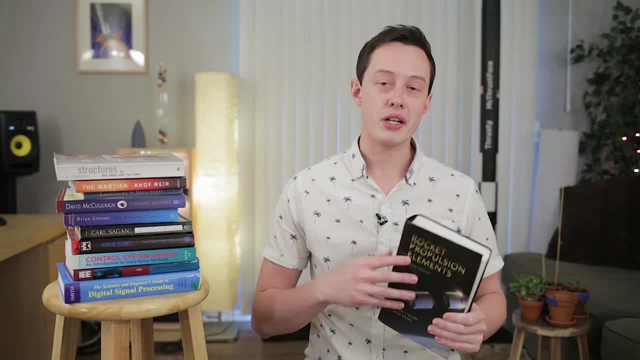 model rocketry, but when I was getting started it was really great for getting a sense, for you know how rockets work and it's just helpful like that. Now there is a bunch of math in here. If you're scared, you can go to the link in the description below. But if you're not scared, 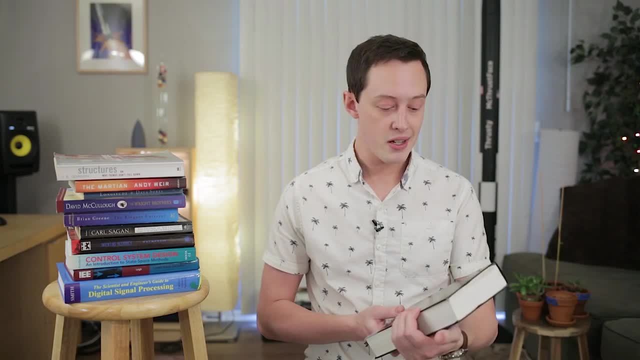 you can go to the link in the description below. And if you're scared, you can go to the link in the description below. And if you're scared, you can go to the link in the description below. It might be a little bit challenging to read, but again it's a super all-encompassing book. 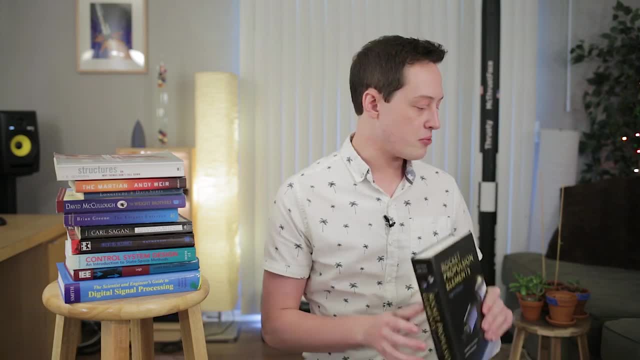 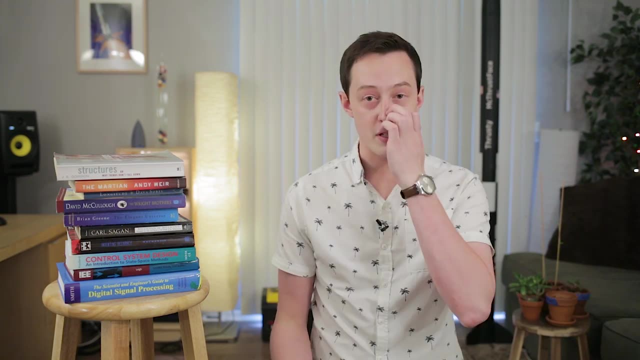 that's a great way to get started. Actually, all-encompassing is not the right word to describe this. It's just a great way to get started. Now the second book that I found helpful when getting started with this stuff. most of you know, I don't actually have a background. 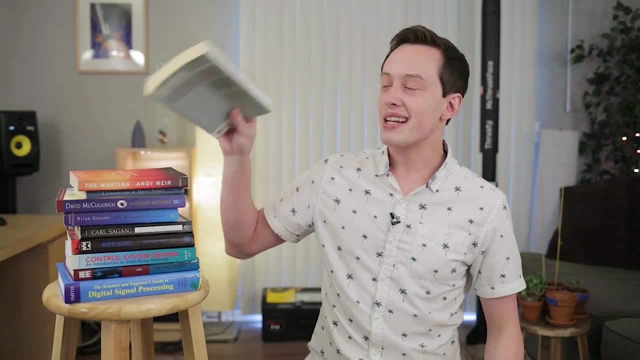 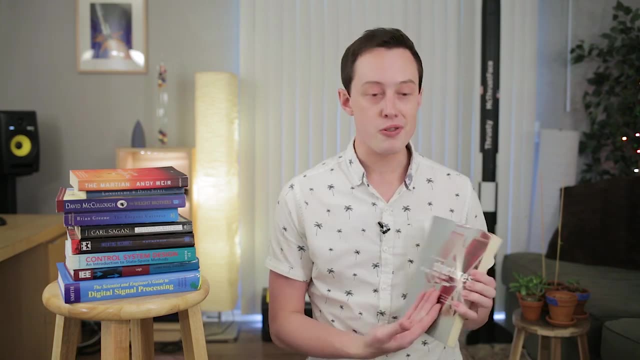 in engineering. I have a degree in music, So in getting started I wanted to learn a little bit more about mechanical engineering, physical design and things like that. So this book called Structures, or Why Things Don't Fall Down, by JE Gordon is an excellent read, And here's. 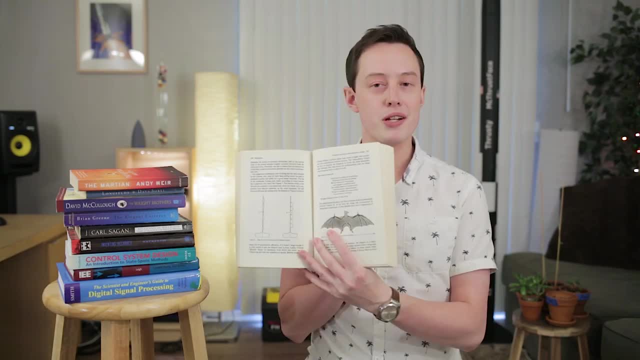 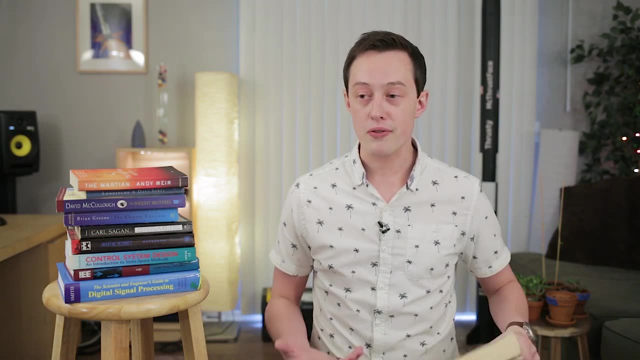 the best part. So this book. there's also cool pictures and diagrams. That's always a plus. There's not a lot of math in here, And so if you're someone who's scared away by math or if you're just starting with no mathematical background, this is a really friendly book to 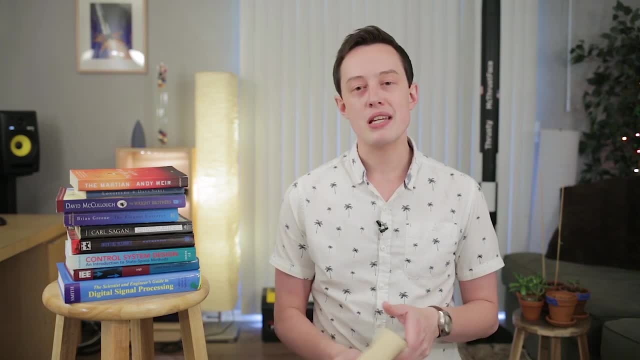 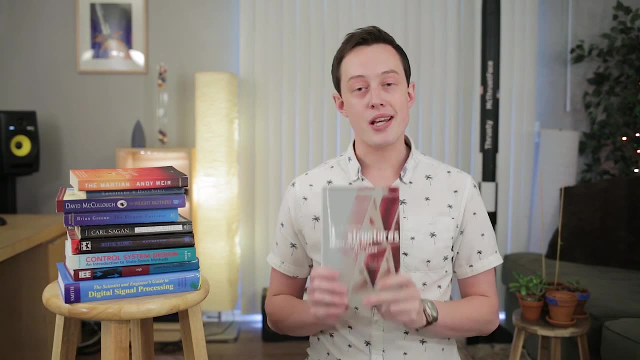 read It honestly is like it's just a really easy read. It's a great way to get familiar with mechanical design And I highly recommend it. So this ends section one of the video, which is basically: those are the two primary books. 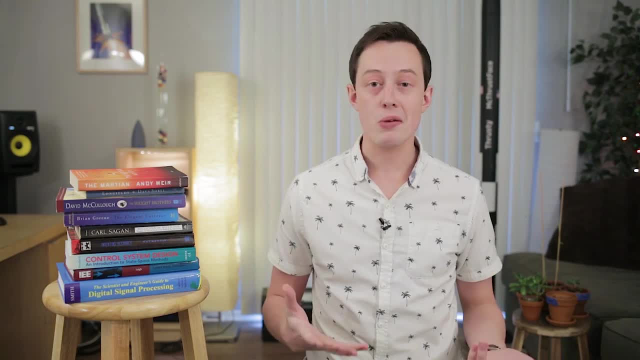 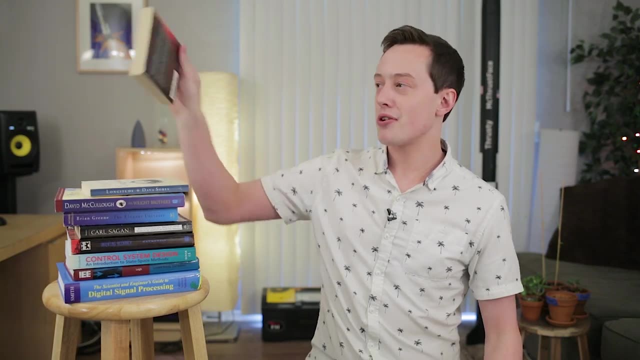 that I used to get started as techs, But I have more recommendations here and I think you'll like them. So section two is books that are sort of engineering focused but are also easy reads, And this is The Martian by Andy Weir. That'll kick us off here. This: 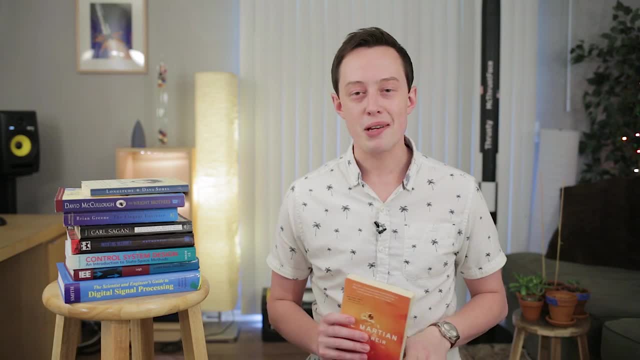 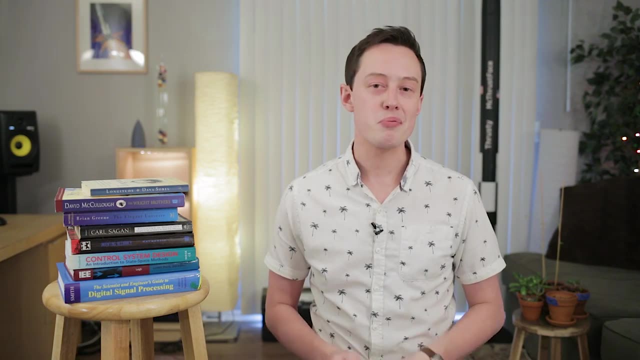 book is awesome. I mean, I would be very surprised if anyone watching this hadn't already read this book or at least watched the movie. But it's a great read And I think it's a. You know, the cliché is true: It is better reading the book than watching the movie. 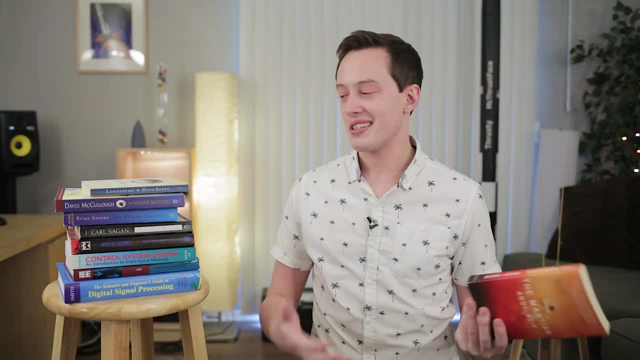 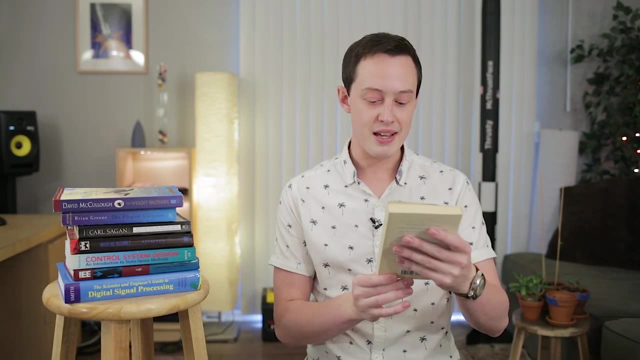 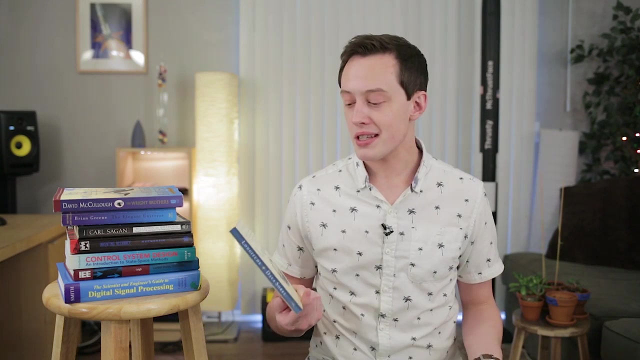 But I highly recommend The Martian. All these things are once again linked down below. Now a lesser-known book: is this guy right here, Longitude by Odeva Sobel. I think I'm pronouncing that right, Longitude is. It's so cool, As with a lot of books in these lists. 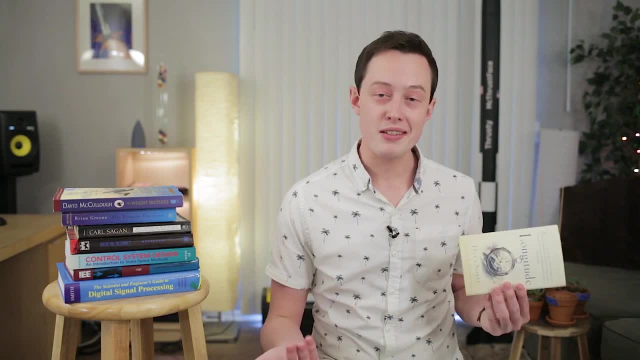 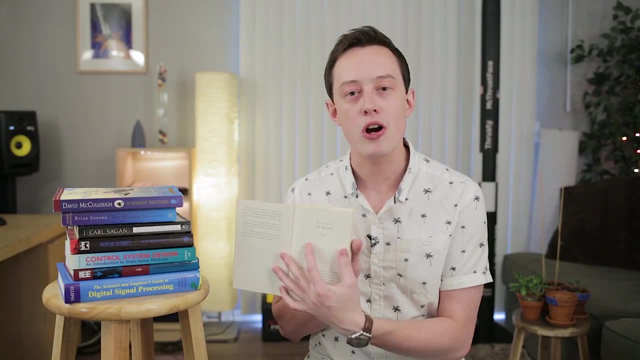 my dad is the person who recommended this book to me, and if this is enough to sell you on it, the foreword in this book. like the, the little starting part, let me just skip to it here. foreword by Neil Armstrong. 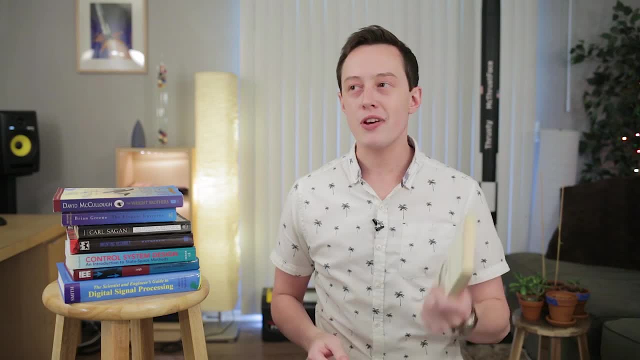 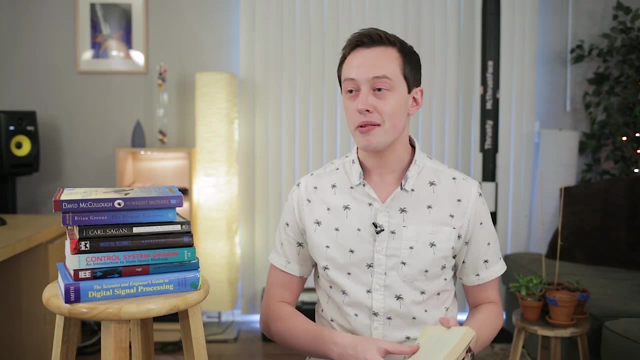 You need this book. You don't actually need it. It's about the development of timekeeping in the in the mid 1700s. So if you can think about the state of machining and precision in mechanical design way back in, you know. 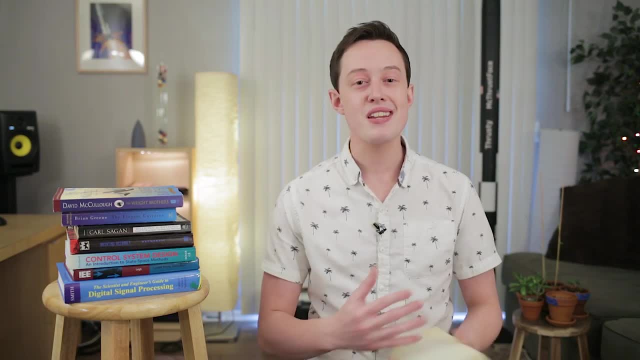 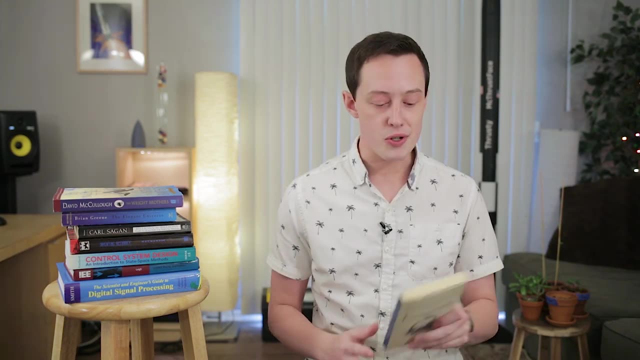 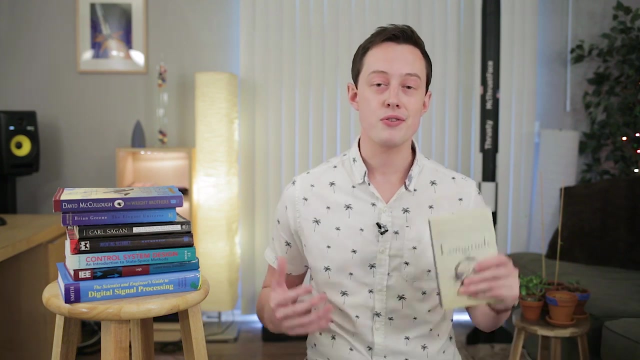 1750 or something like that, you have to imagine that we don't have nearly the control over precision measurements and precision timing. It's about timekeeping specifically back then, And so John Harrison is a gentleman who developed Basically. he dedicated a ton of time in his life to developing accurate timekeeping at sea for boats. 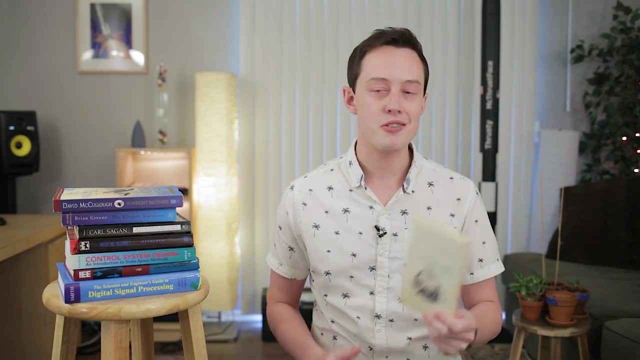 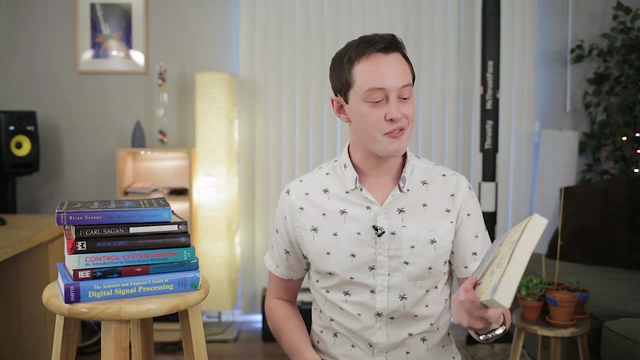 I won't give too much else away. I mean, it's it's basically a history, but it's a great read. I highly recommend it. Next up is The Wright Brothers. This book is awesome. Another recommendation from my dad, and the reason he recommended it to me is he realized when he was reading it that they test in. 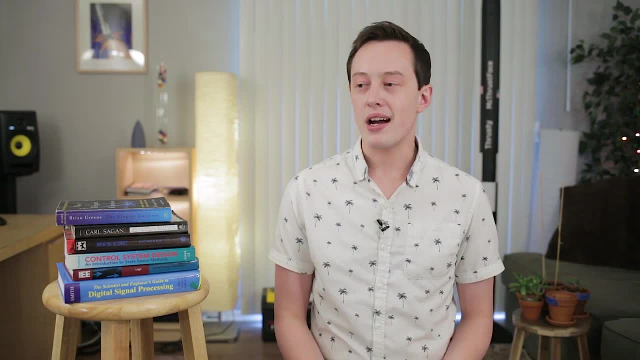 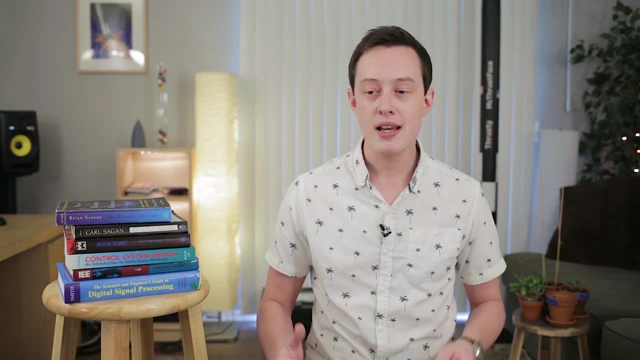 the same way that I used to test my rockets. So I, especially at the beginning of BPS, I tested a lot of things very privately. I didn't invite people to launches, I did. I basically only invited like a couple of really close friends. but 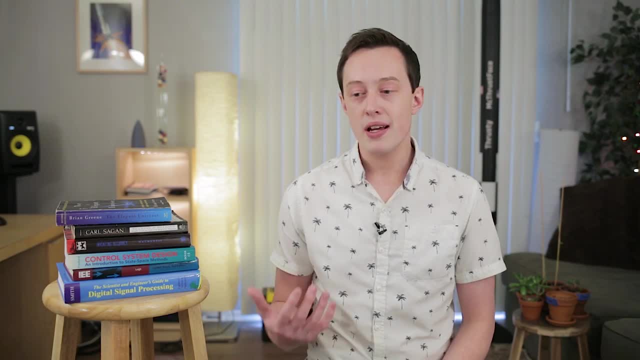 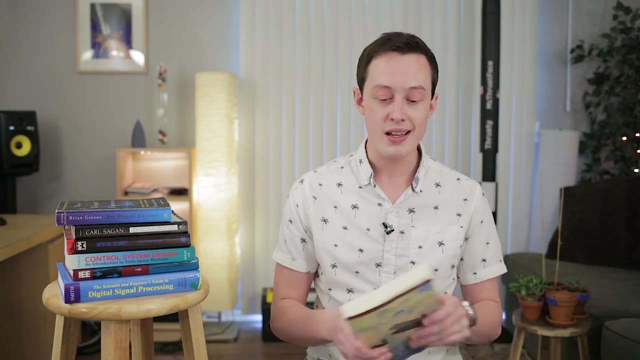 it's a thing that I still do for some of the testing today, where I just try to keep stress low and publicity low for a lot of these things, because it helps me test and stay focused on the hard science and the hard data, And the Wright Brothers do the exact same thing in this book. 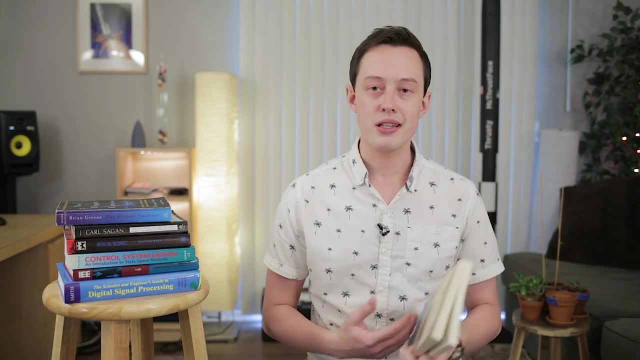 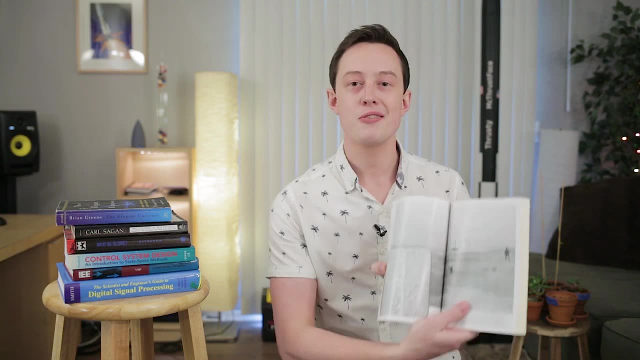 So this is a documentation of how they went about creating the first flying craft and I do highly recommend it. There are cool pictures in here. A lot of these books have like neat pictures, but it's a great basically account of their progress and 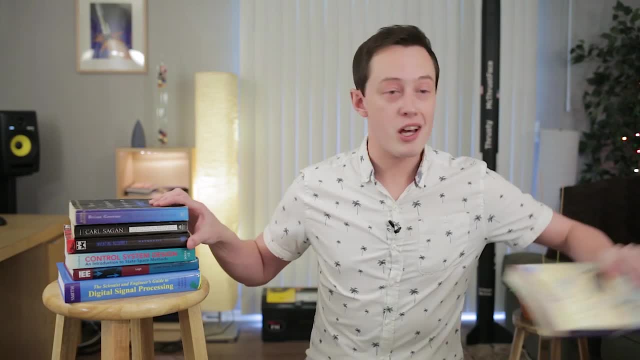 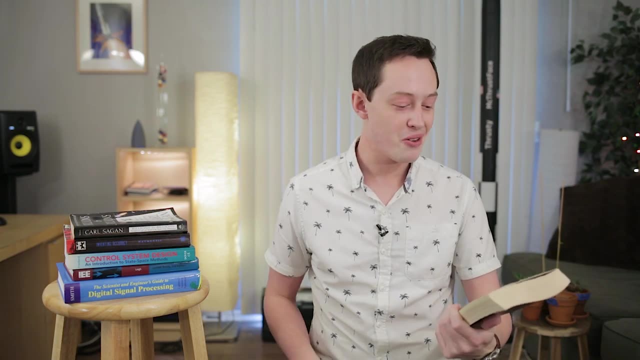 their struggle through developing these flying craft. Next up is The Elegant Universe by Brian Greene. I actually did not finish this book, but I do recommend it. There's only a finite amount of time in my day, and so this book is about string theory. 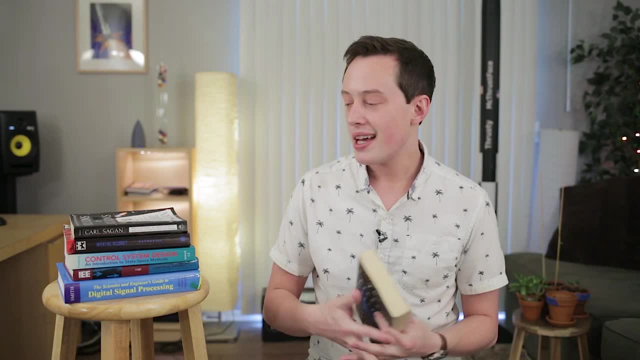 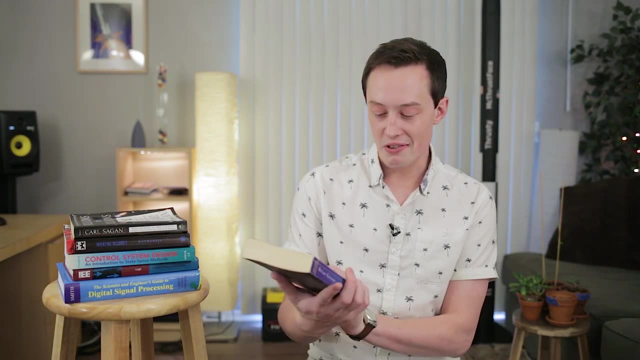 theory and a lot of stuff that happens at the really small level, and I do recommend it. I just wish I had time to finish it too. this is, I guess, I guess a sort of half recommendation, because I wasn't able to finish this one, but on the cover it says super strings, hidden dimensions and the 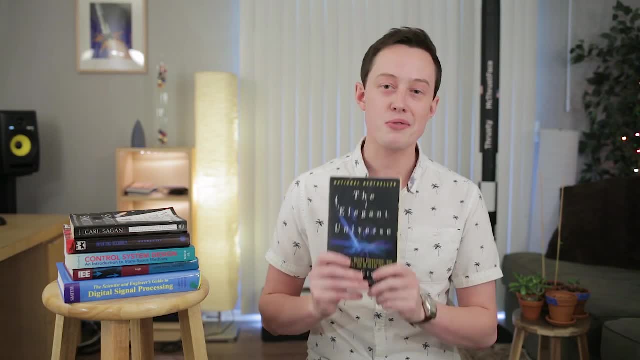 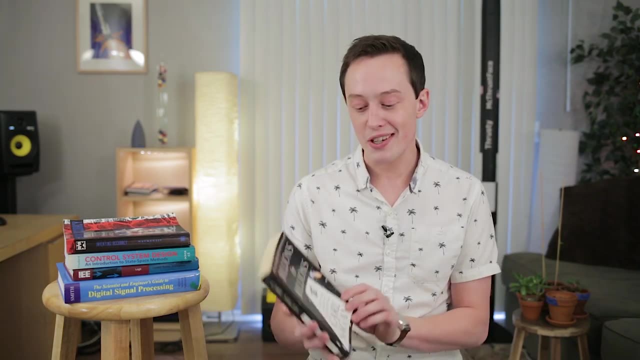 quest for the ultimate theory. I do really like it, though, so it's a recommendation. it made the list. now, the next thing that made the list makes the list so hard. like it, just it's so good. billions and billions by Carl Sagan. I think most of you have probably read this as well, but if you haven't, 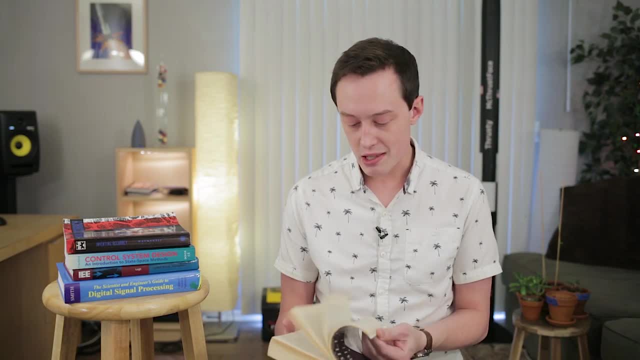 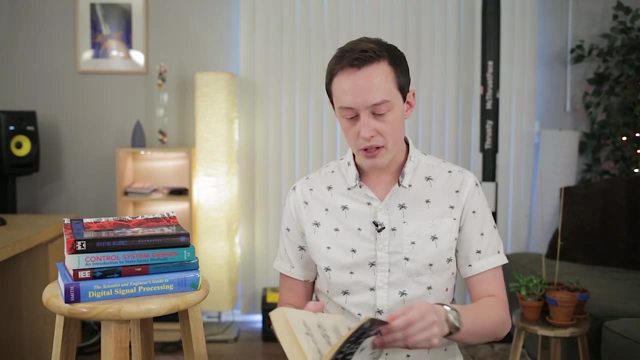 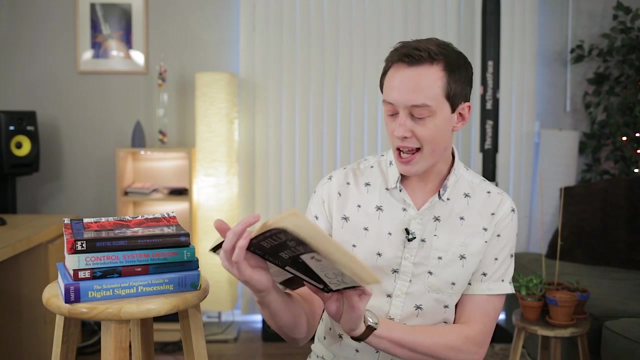 please, please do. my favorite part about this book is at the beginning of it. um, oh man, do you think I can skip to it in real time? at the beginning, Carl puts this brilliant diagram of the electromagnetic spectrum that, like helped solidify in here. it is okay, it helped solidify in place in. 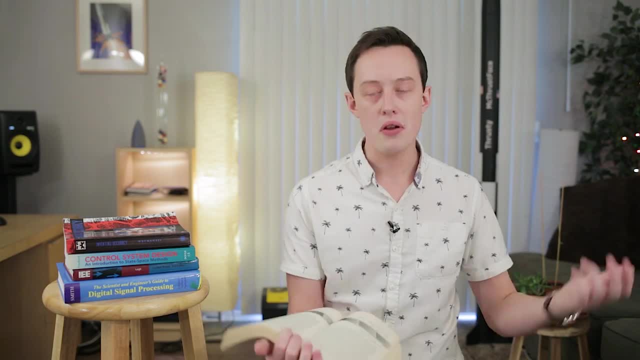 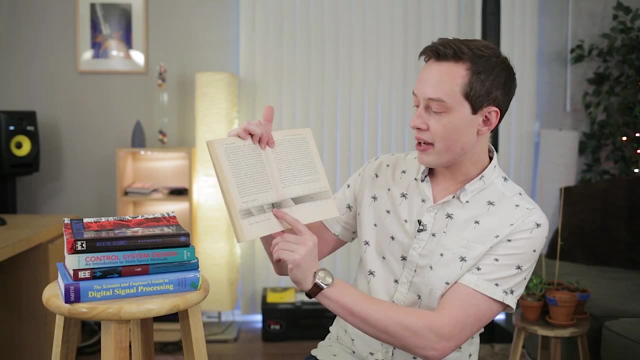 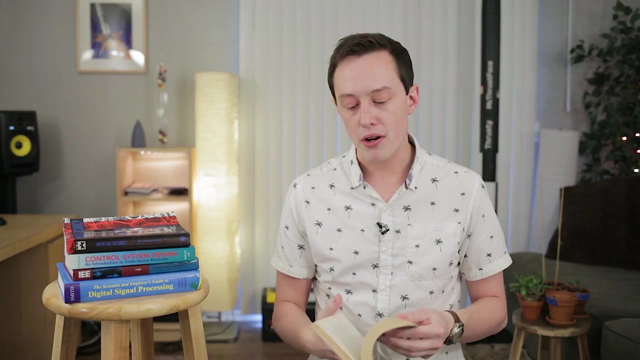 my mind how light, um, and radio and all of these things are interconnected. so this is basically wavelength in centimeters and you go from gamma-ray to x-ray, to ultraviolet, to infrared, to radio, and right here this is just a tiny visible spectrum. um, this book is about all sorts. 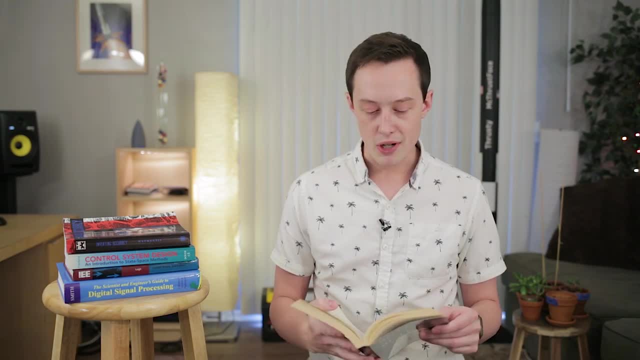 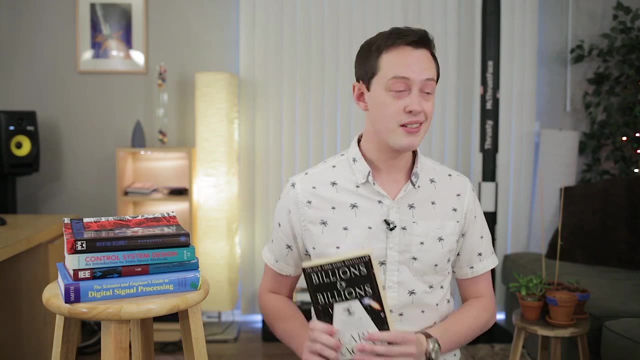 of things, that he talks a little bit about climate change in it as well. um, Carl Sagan is a brilliant mind and was a national treasure, so I recommend reading this. it's, it's all around excellent. the next book in our list and the final in the list of sort of personal slash engineering books is: uh. 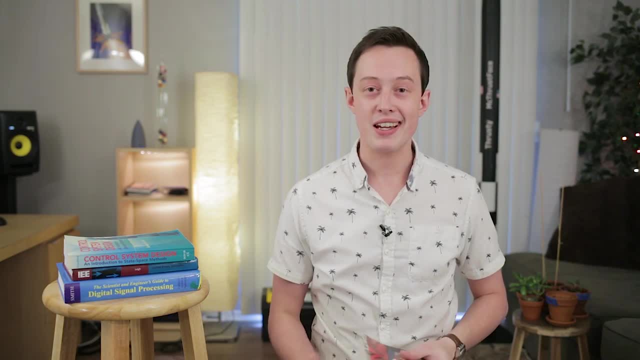 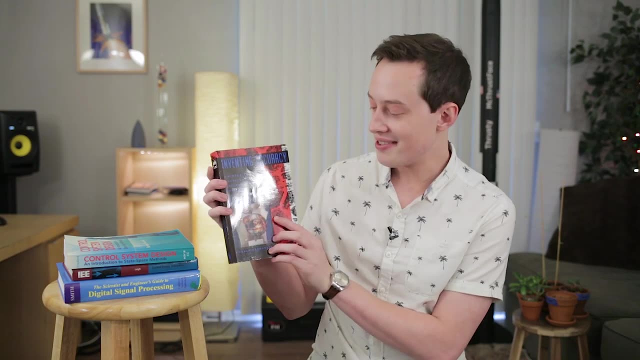 well, it's a little bit of a long list. but it's a little bit of a long list but it's a little bit spicy, but it is really good. it's called inventing accuracy and the subtitle is a historical sociology of nuclear missile guidance, and on the front here you can see someone dealing with um a. 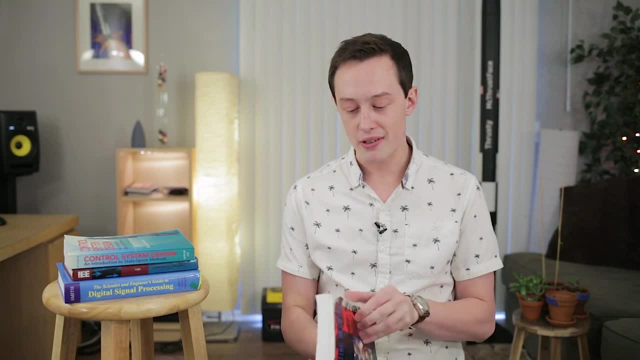 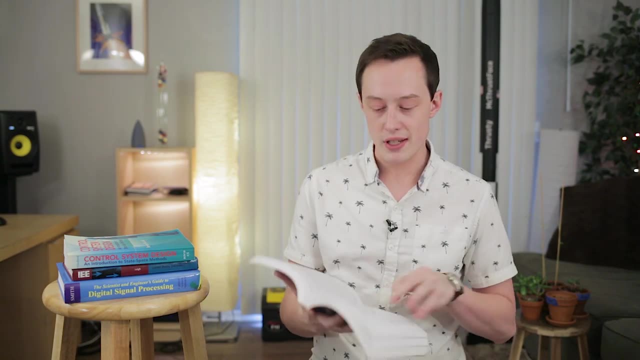 an IMU from way back when for the peacekeeper, uh, missile. anyway, this book is. I originally bought it because I found a lot of diagrams online that I thought might be interesting. so here's a diagram of ballistic missile stellar inertial guidance system. um, there's, there's diagrams of 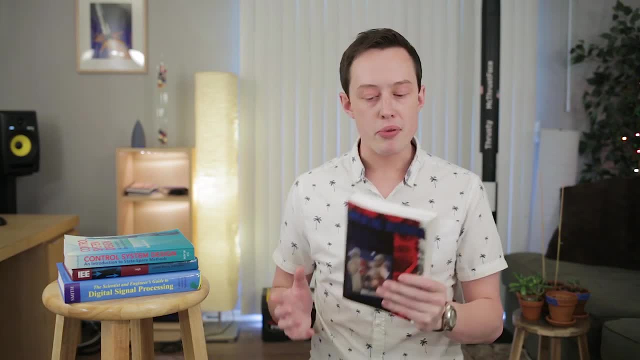 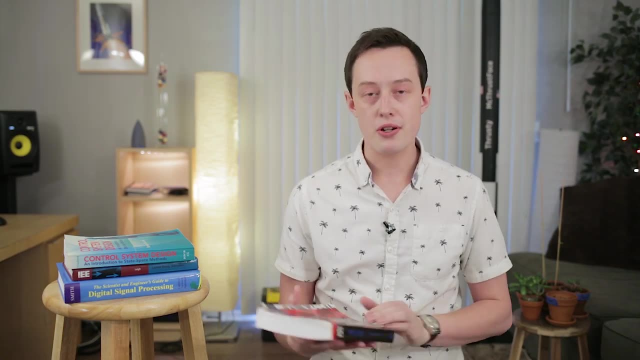 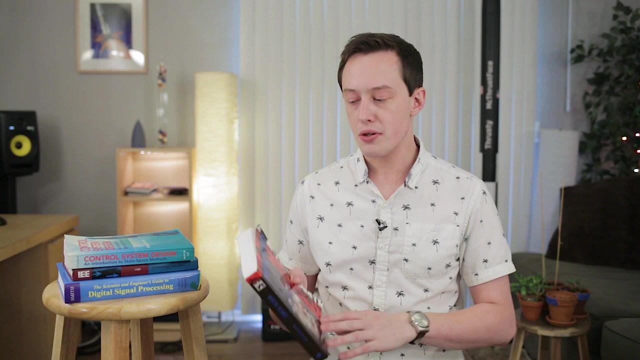 early, uh, gyroscope development and things like that. um, but it's really about the sociology of doing what people thought was impossible for a long time. so, um, Charles Stark Draper of the of Lincoln Labs and MIT headed a lot of the development of um, basically nuclear missile. 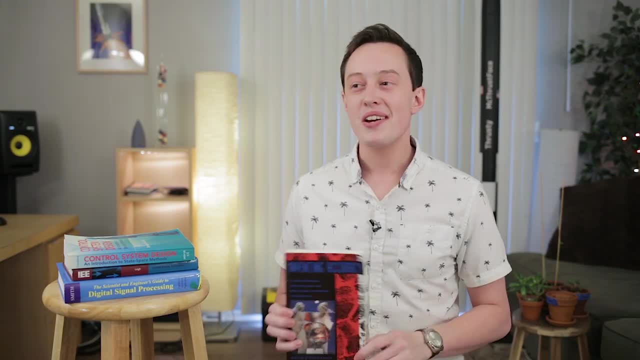 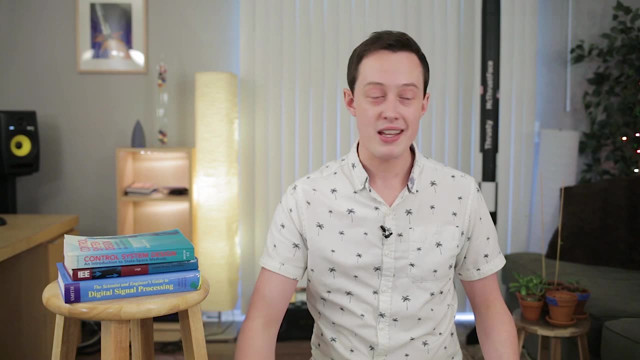 guidance and I don't love nuclear missiles that much um, but mostly a lot of the technology that's used in them is the same technology. this is very topical because of the 50- 50th anniversary of it. it's a similar technology to um, the Apollo guidance computer and the guidance system for 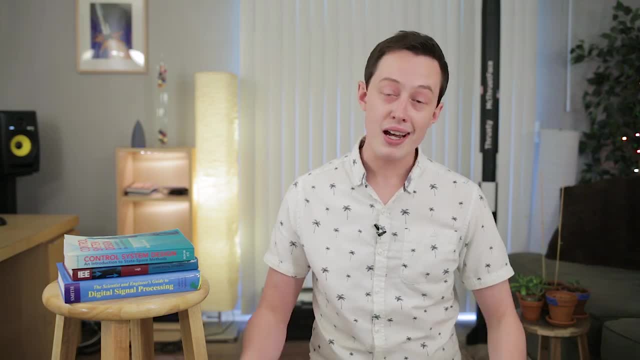 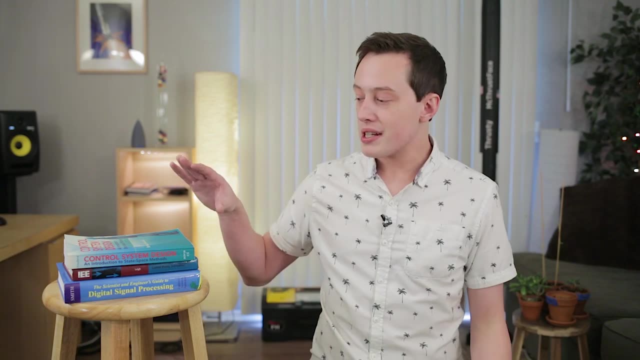 the Saturn 5, so I picked up this book mostly for that, and I do recommend it. it's a great read. now we've reached the third section of the video, where I want to talk about the books that I'm reading right now, and there are just three here. the first one is called control system design: an introduction. 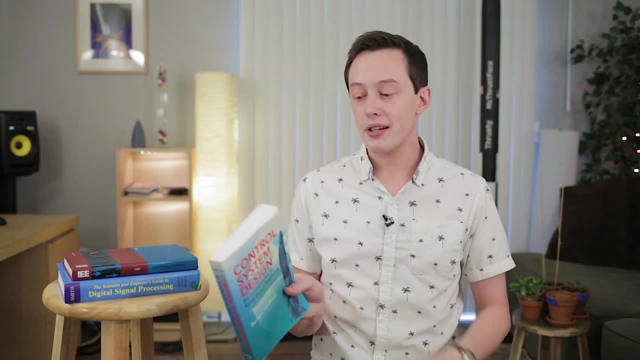 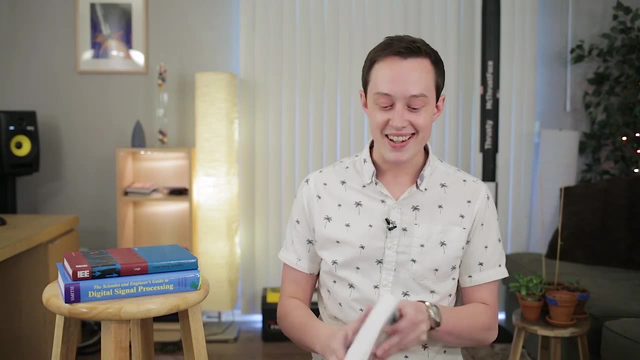 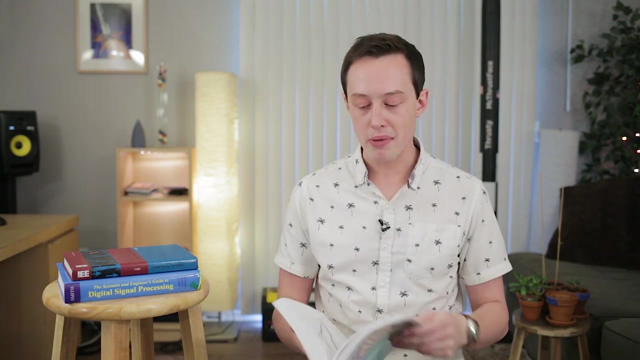 to state space methods by Bernard Friedland. this book is dense. if you don't have a solid background, uh, it's going to be really hard to read. there's a there's a tremendous amount of math here, there are some cool diagrams and it's. it's basically about control system. I mean, it's a control system. 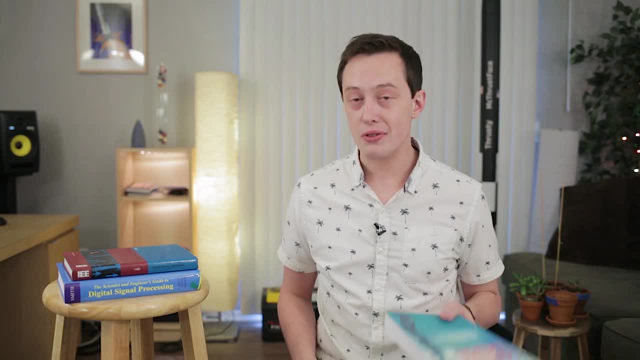 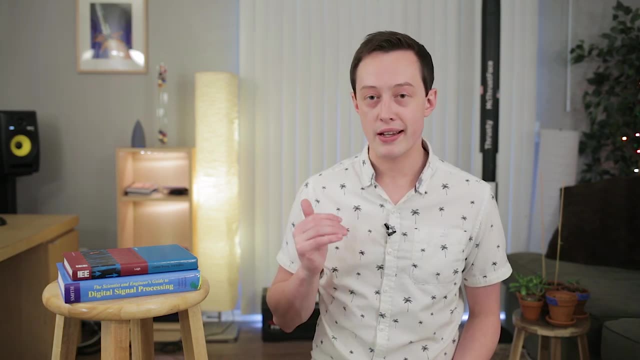 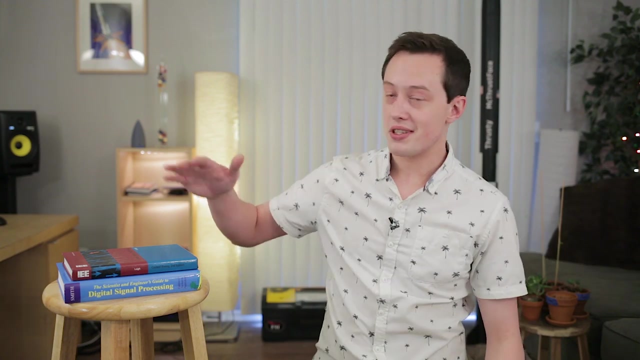 design. but, um, I do recommend it. it is a great read. it's just one of those books that you have to read every page three or four times and you can't expect to like just chug through it, unless you're really well grounded in control systems. and if you're not really well grounded in control. 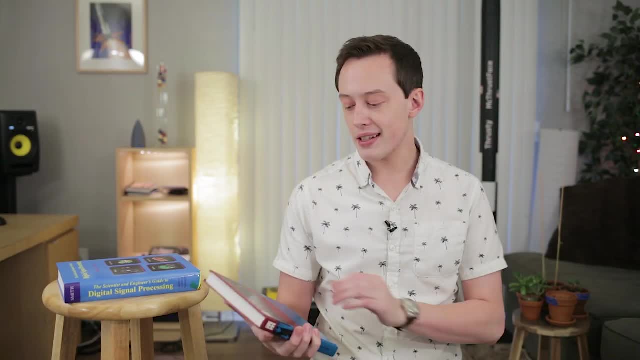 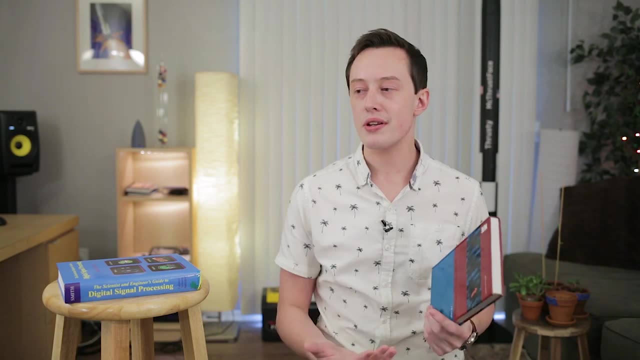 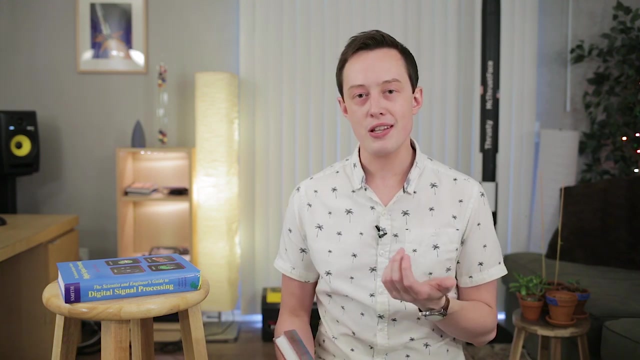 systems. here you go. control theory, second edition by JR Lay. there are a lot of books that are general, basically overviews of control theory, and control theory is used everywhere in the world for all time. but control theory is really the heart of how do you spec out your PID gains? how do you decide? 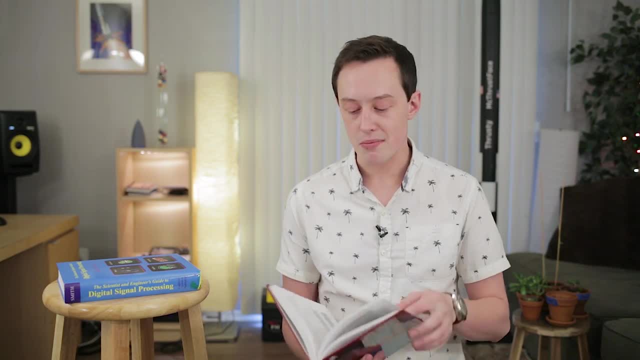 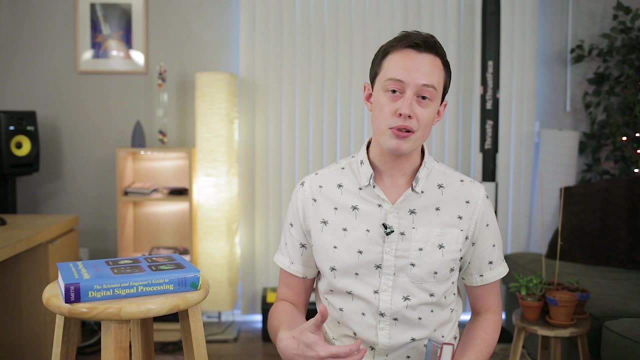 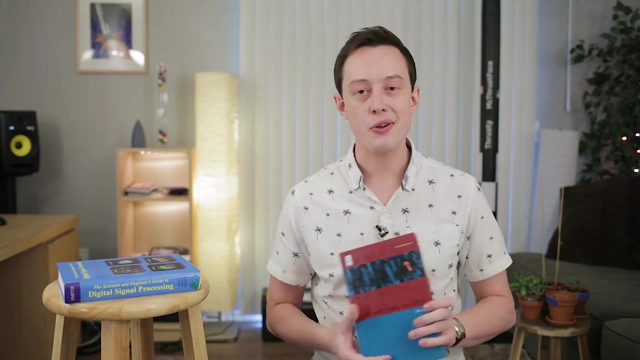 if your rocket is stable or not with an active stability system. so this book is an excellent introduction. it was recommended to me by Brian Douglas of control system lectures. his YouTube channel is linked down below and it's a video full of recommendations. but you should check his- his, uh, his- YouTube channel out. so control. 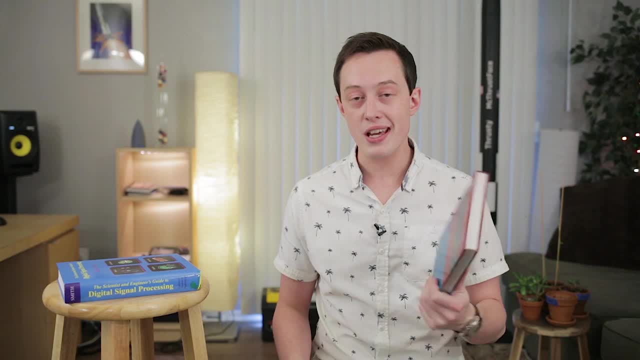 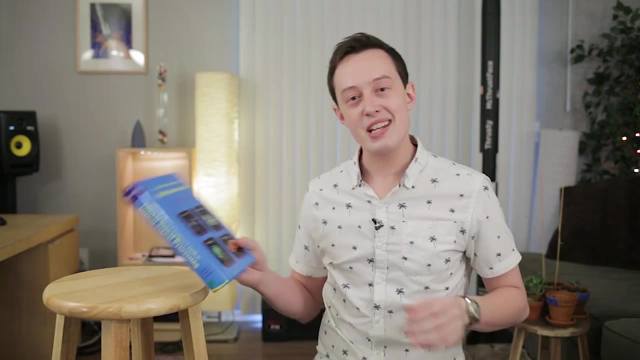 theory second edition. I'm really liking this so far. I have not finished it yet, but it's a very friendly introduction to control systems and it's been valuable for me for sure. the last book that I've got here is dense. this is a heavy book called digital signal processing by Stephen W Smith, and 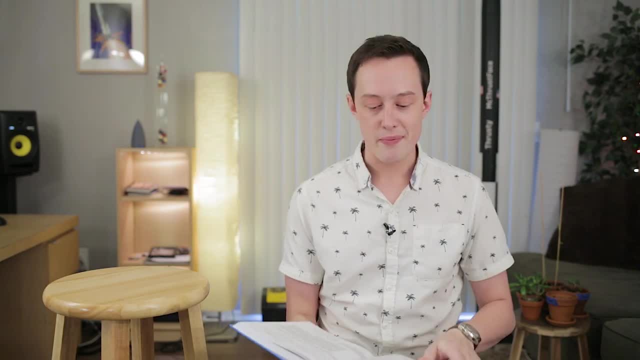 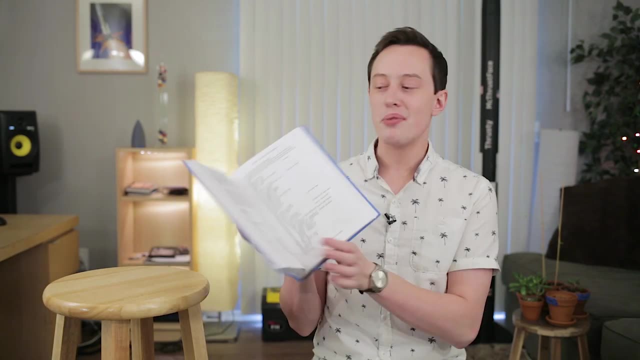 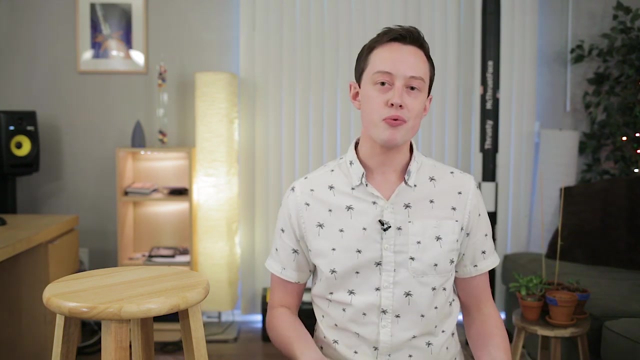 this is a book on, well, exactly what it sounds like. DSP, um, DSP, just like control systems, is used everywhere. it is- look, it's got some code in here. I think this is Fortran, um. but yeah, DSP is used everywhere and it's just how. it's how your signals get analyzed. it's how we sense things on mems. 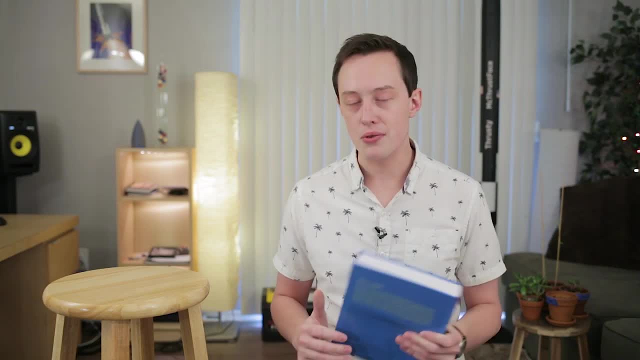 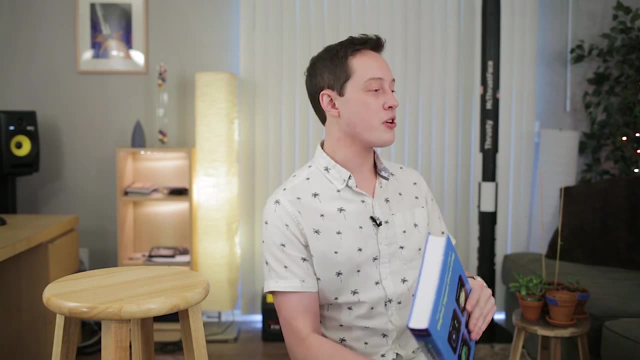 accelerometers and gyroscopes. I mean there's no way to all-encompassing describe how valuable this book is in describing all of these systems. so that's a very wordy way to say I recommend it. and that brings us to the end of my recommendations for sciency and engineering. 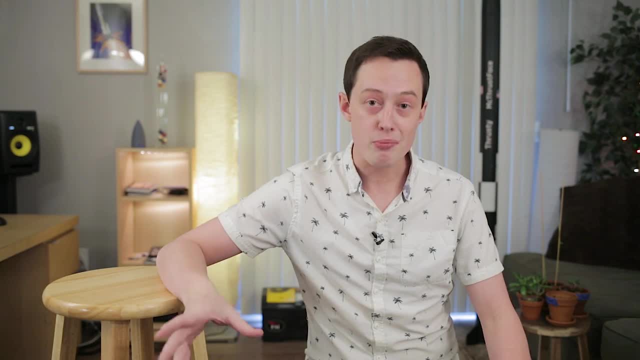 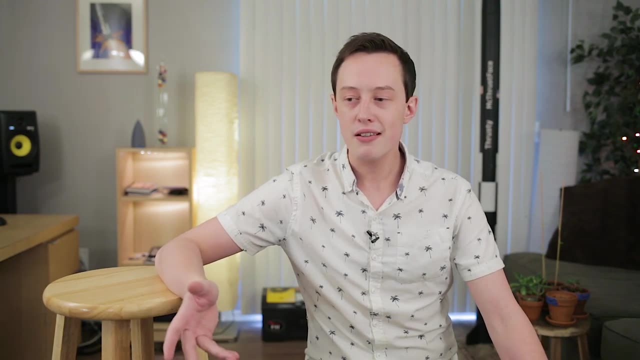 books. I've got another list of recommendations for more personal books on the second Channel, um, and this is actually the first video in a set of, I think, two videos that I will do so the second video is going to be online resources that I felt found helpful. you don't just want to. 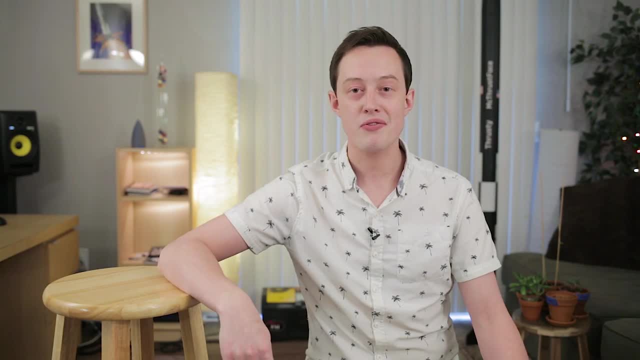 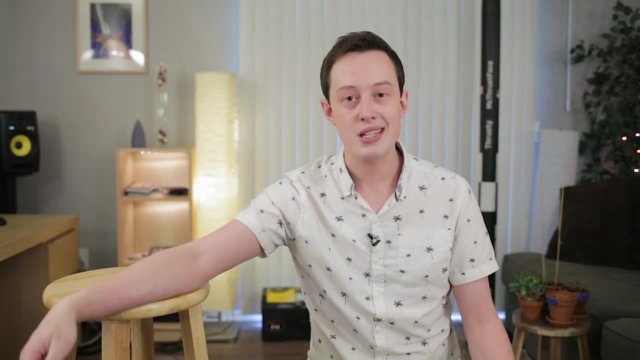 read books. you want to learn how to code. I mean, learning how to code from a book has got to be very hard. I didn't do it that way, so I'm going to do a video on online resources that I found helpful and that I still use today, and these are all basically centered around 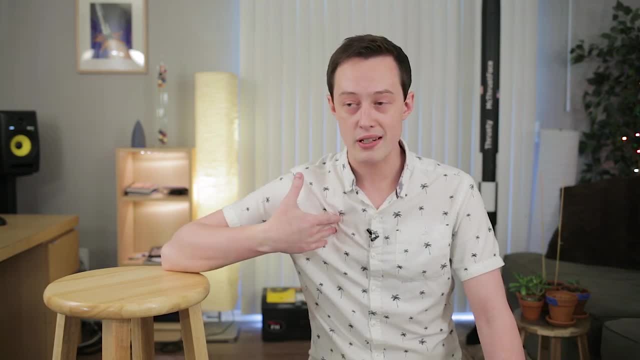 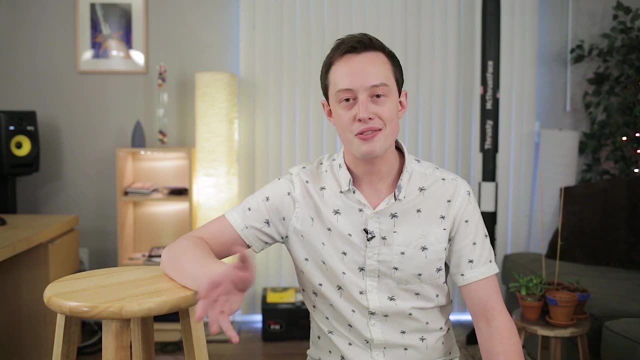 what I can personally vouch for and what I personally used in learning and getting started with BPS. so I know this is a little bit of a departure from the normal style of video- either launches or tests or things like that- but I like to keep experimenting with what works and 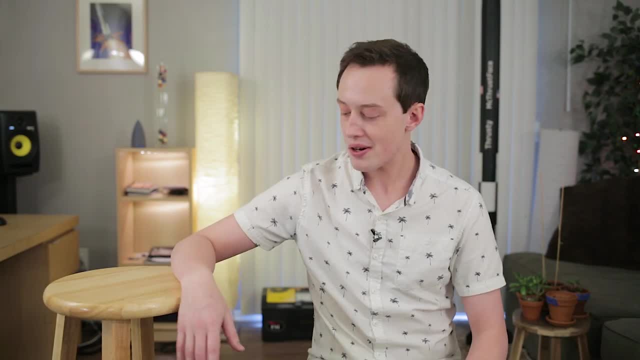 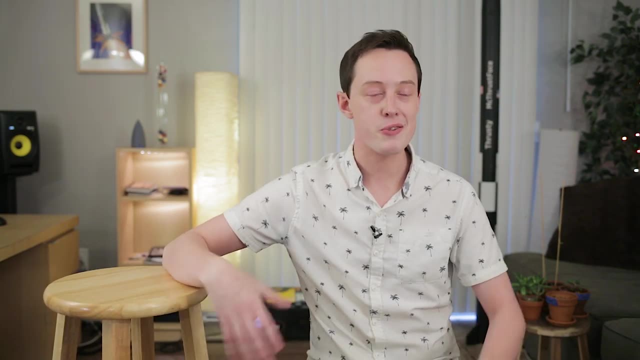 what doesn't on this channel, so thanks for being patient if this wasn't your type of video. we've got a lot of cool stuff coming up soon and I think that's it for now, so thanks again to the folks on Patreon who support this project and make it all possible, and 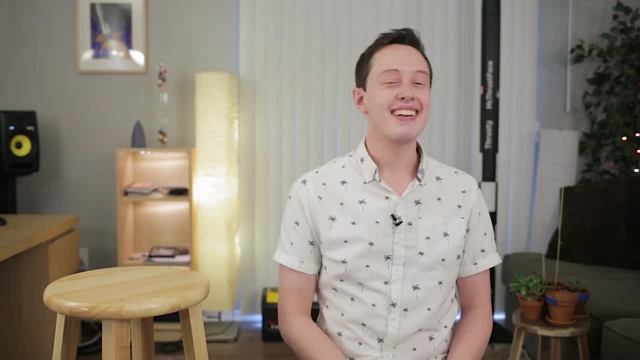 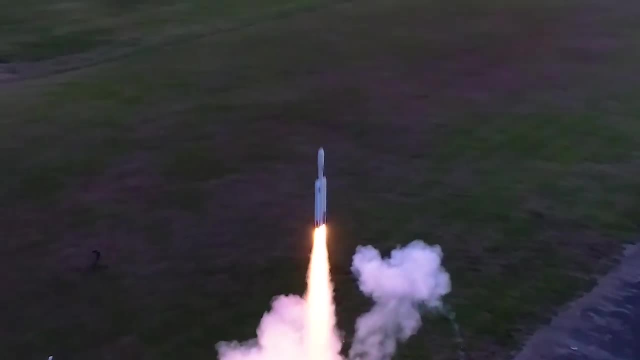 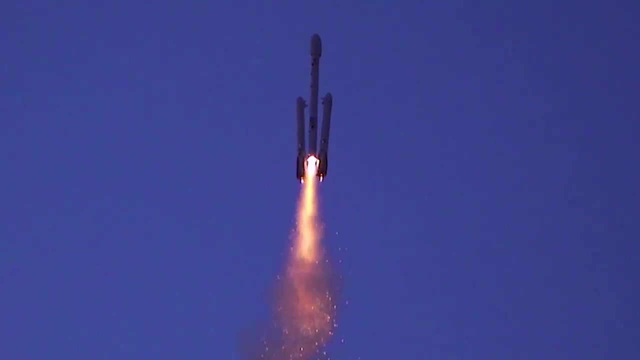 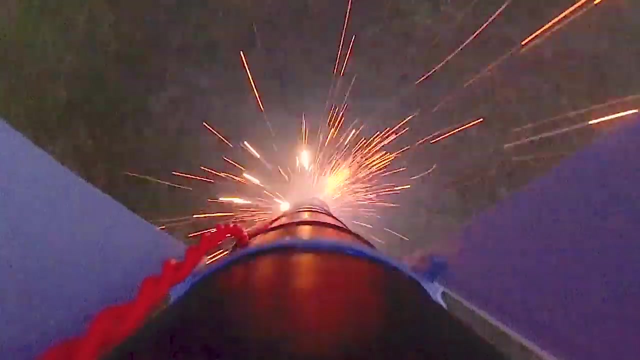 that's all for me for now. all right, goodbye everyone. may your skies be blue and your winds be low. you.